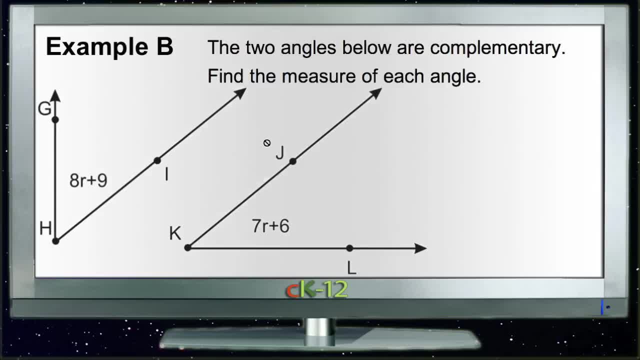 Example B again tells us that the two angles we're given are complementary, but doesn't actually give us any degree measure for either angle. All we have is an expression that tells us that the number of degrees in the first angle is 8R. 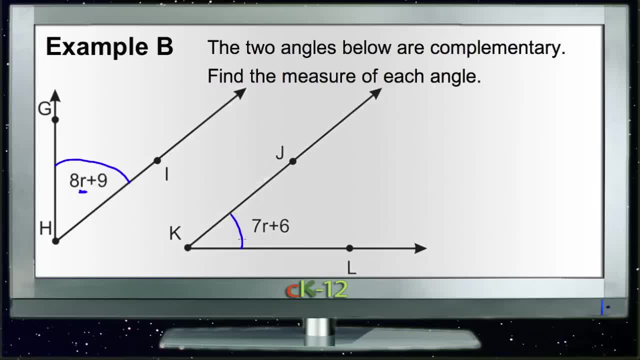 some unknown variable plus 9 degrees, And that the second measure is 7R- the same variable plus 6 degrees. That tells us that whatever R is going to be, it will be the same thing in both measures. But we don't know anything about the degree measure of either of these yet. 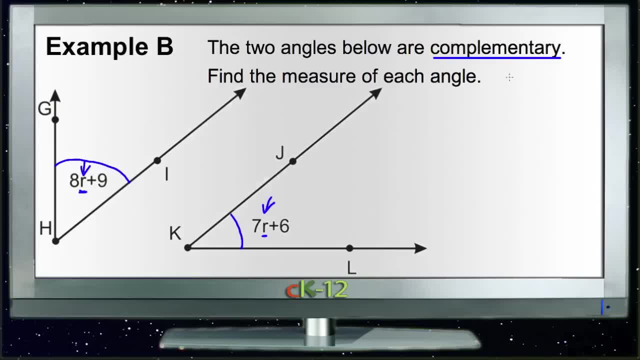 However, we do know that the angles are complementary. So the total of the two angles together must be 90 degrees. So if we add the two angles together, 8R plus 9, added to 7R plus 6, that total has to be 90 degrees. 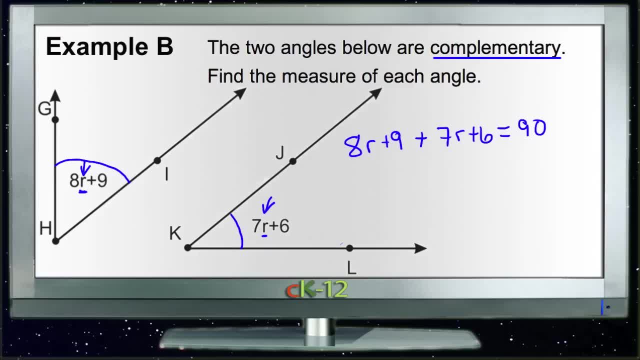 Then we can just combine like terms- I'll do that in a different color so that they show up a little better for you. So we combine like terms: 8R plus 7R gives us 15R, And then 9 plus 6 gives us 15.. 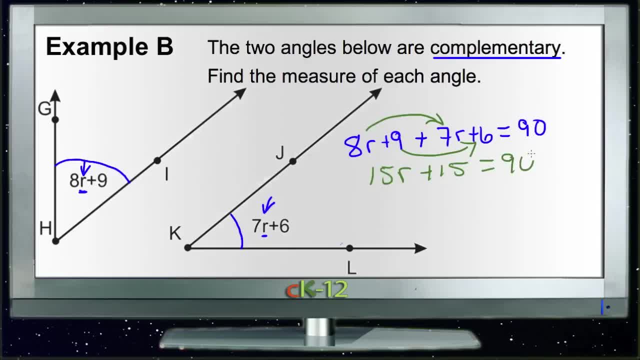 We know that that equals 90 degrees. Then if we subtract 15 from both sides, we'll have just 15R on the left-hand side and we'll have 75 on the right-hand side If 15R equals 75, then we could divide everything by 15,. 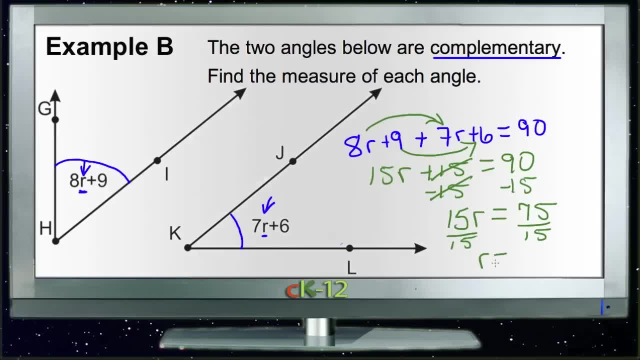 and learn that R must be 5.. If R is 5, then since the first degree measure is 8R plus 9,, it would be 8 times 5 plus 9,, or 40 plus 9,, or 49 degrees. 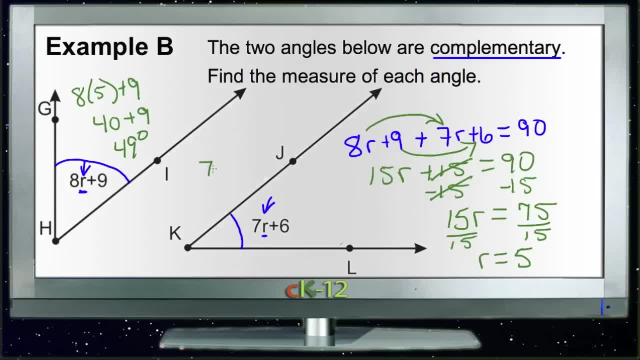 The second angle measure then would be 7 times 5 plus 6, or 35 plus 6, or 41 degrees, And since 49 plus 41 equals 90, we know that our two angle measures are correct. So you can see that you don't even have to have any degree measures at all.